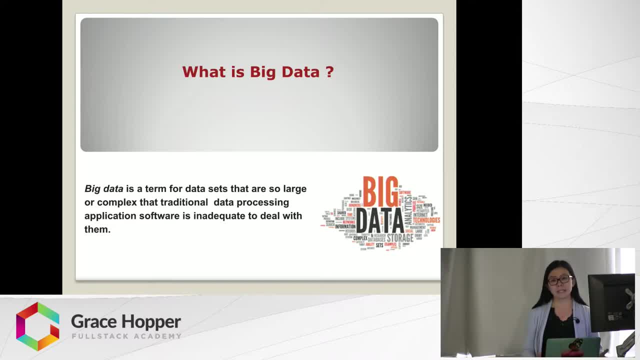 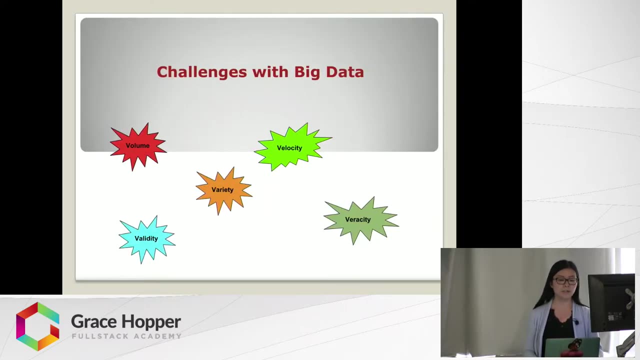 Big data is just a problem statement. It is actually a term for a data set that is so large and complex that traditional database system is not able to handle it. So working with big data also involves a lot of different challenges. So working with big data also involves a lot of different challenges. 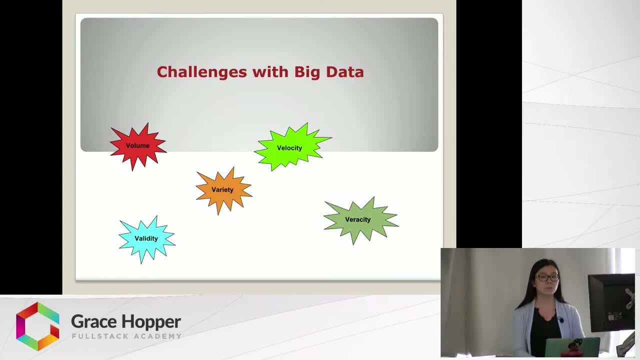 It's not just about the size. it can be the variety, which refers to the fact that data is coming from different sources in different formats. Also, the velocity refers to the fastest speed that data is generated. So in the past we have been using relational database management system to deal with our data. 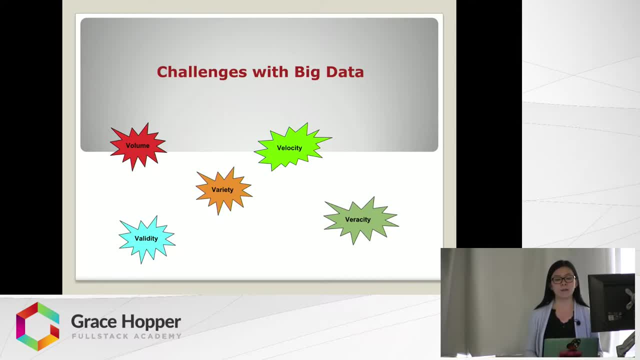 But one big issue with that is that today a lot of data is semi-structured and unstructured at all, So which means all those data is going to be very hard to fit into our traditional predefined models. So obviously traditional database is definitely not going to be a solution for our big data issue. 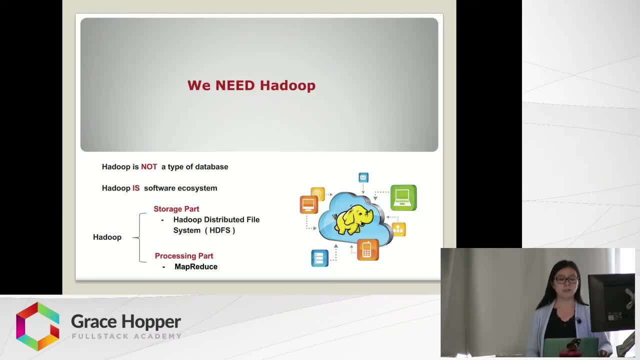 So here that's why we need Hadoop. Actually, Hadoop, as we just mentioned, definitely not one of those traditional database. It's actually a data software ecosystem that allows for massive parallel computing. Hadoop actually is an open source software framework written in Java. 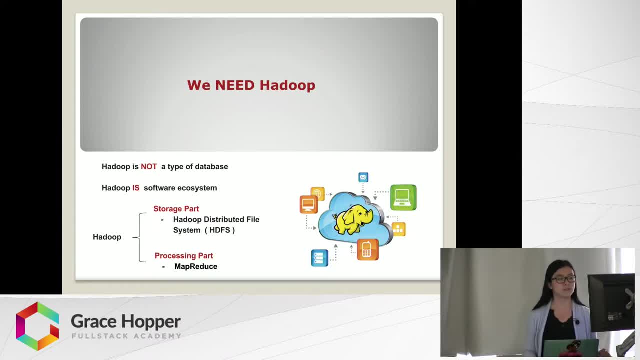 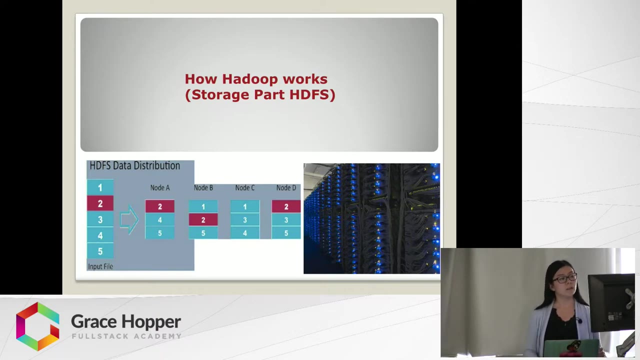 Also, it has two important parts. One is the storage part on Hadoop distributed file system, HDFS. The other part is the processing part, which is called MapReduce. So let's see how HDFS works. When we have a lot of data coming in, we can split with Hadoop HDFS system. 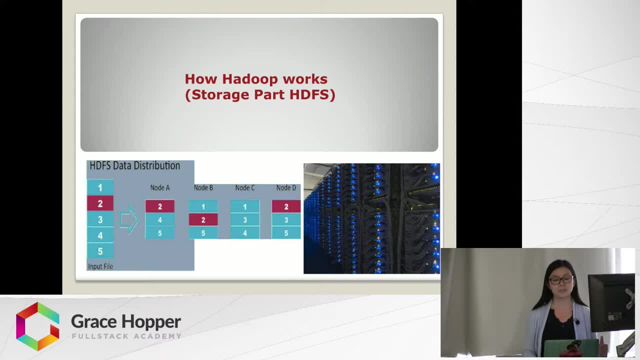 It will allow us to split the data and store them across a collection of different machines, which is also called cluster. Then we want to process the data, Since the data is already stored in the machine, so we don't need to retrieve it from the server, which can be very efficient. 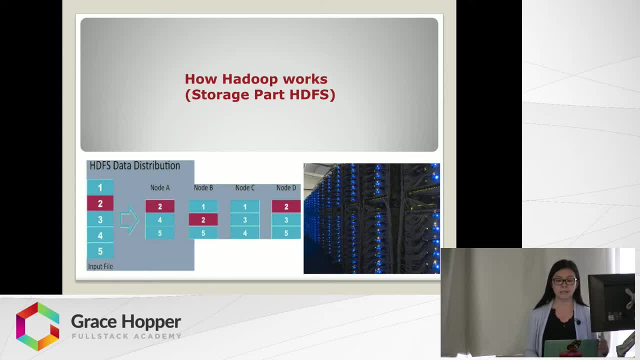 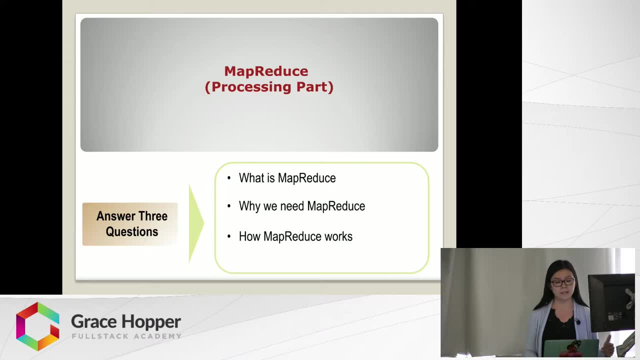 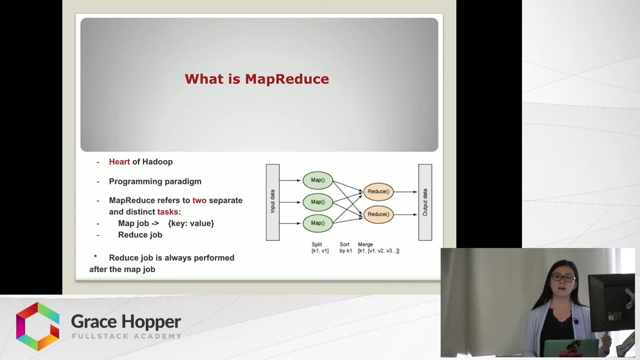 We can process it locally in our machine instead, which can be much faster. So after the data is stored in HDFS, let's see how it's processed with MapReduce. So MapReduce is the heart of Hadoop. It is the programming paradigm that allows for processing large data set in distributed fashion over several machines. 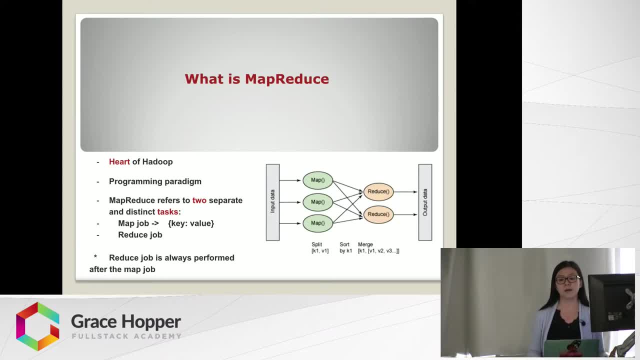 Also, it can be hundreds or thousands of Hadoop cluster. Imagine we have a huge file and processing it in a traditional way is going to take a lot of time, So we are going to divide all those huge files into small chunks, then process the data in parallel. 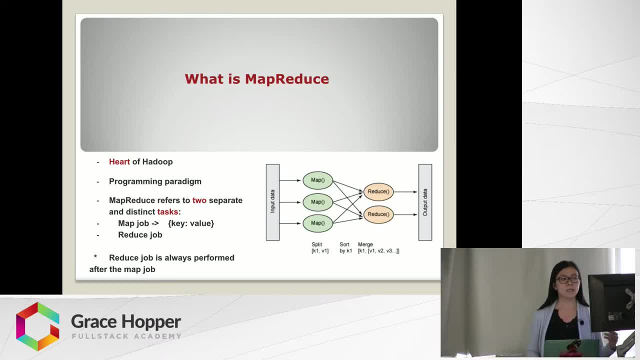 The cool idea behind MapReduce is that we can map all those data into key-value pairs And then the reducer is going to take the output from the map and then combine all those data values with the same key and then process it as needed. 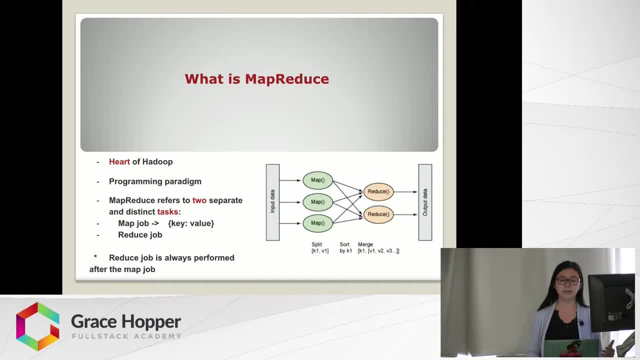 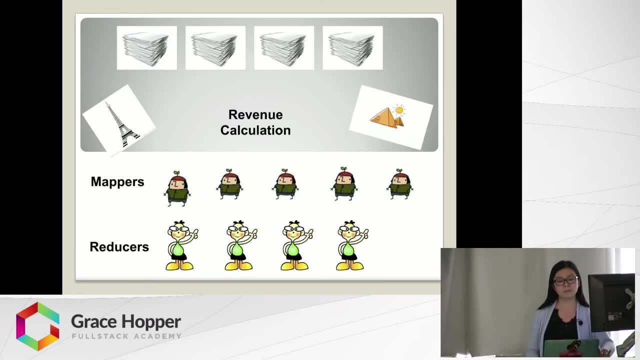 So, as the sequence of the names, MapReduce implies the reduced job always performed after the mapped job. So let's look at one simple example to see how MapReduce works. Imagine we are a big company and we have entities in thousands of different cities. 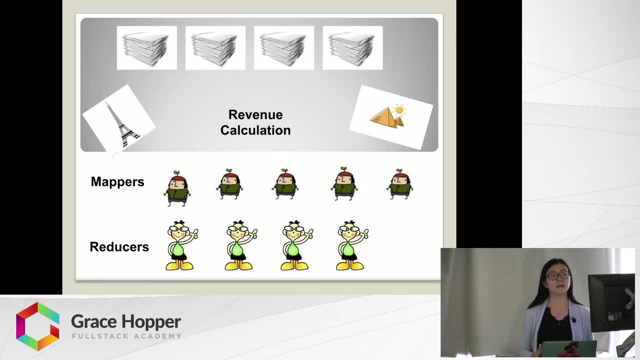 And right now we have a huge accounting journal ledger in front of us including all the sales transactions in all the entities around the world. So our task is to calculate the revenues and sales in each city. So if we go through all those transactions line by line, it's definitely going to take a lot of time. 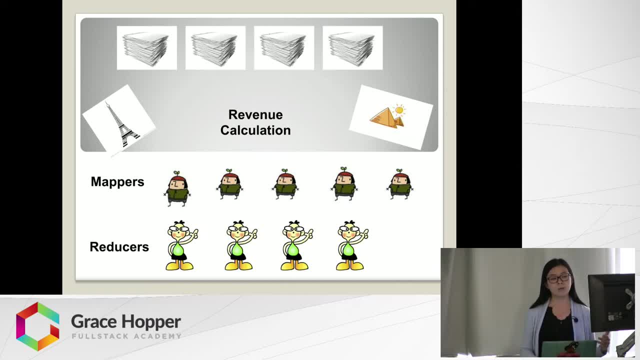 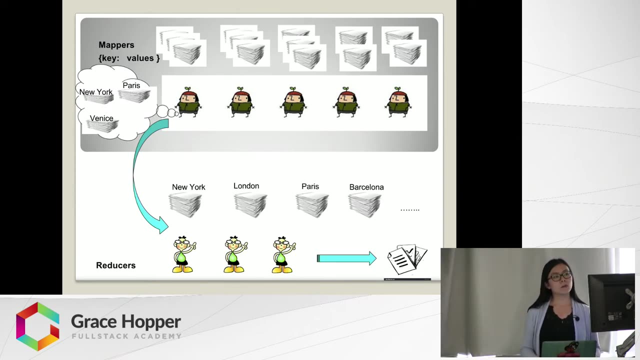 So, given that it's going to be a huge task, we will call more people to help us out. We divide these two groups of people into the mapper group and the reducer group. Let's see, with this huge sales data, we will break it into several stacks. 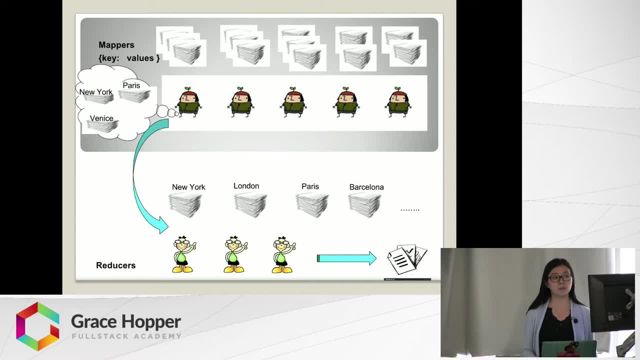 and give each mapper several piles of documents for them to work with. So, for each mapper, we expect them to map all those data according to the name of the city, which means in the end, in front of each mapper, we expect to see several piles of documents. 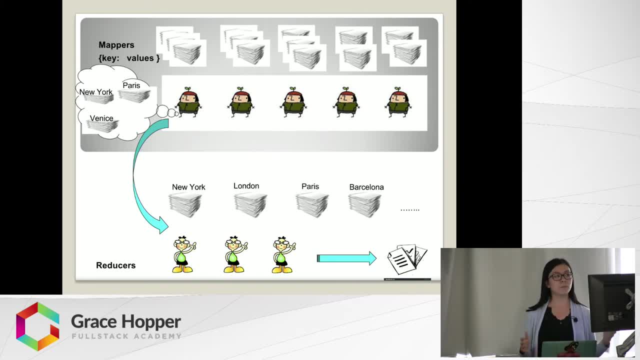 Like, for example, for the first guy. he's going to have several piles: one pile for New York City, one pile for Paris, which means all the transactions happen in Paris. He's going to gather all those data and put them in the same pile. 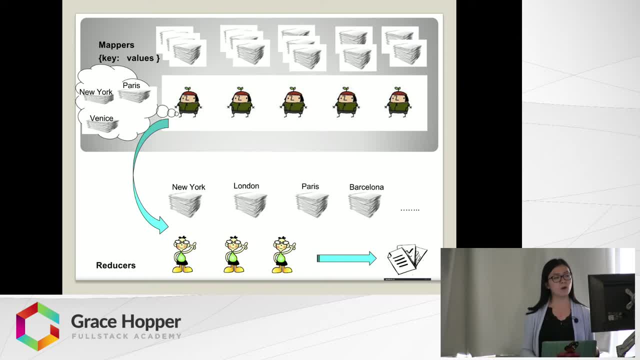 So after the mappers finish working, we are going to call for help from the reducers. Their job is to make sure there will only be one pile for each city. So in the end, like what we see from the slides, we will see only one huge pile for New York City transactions. 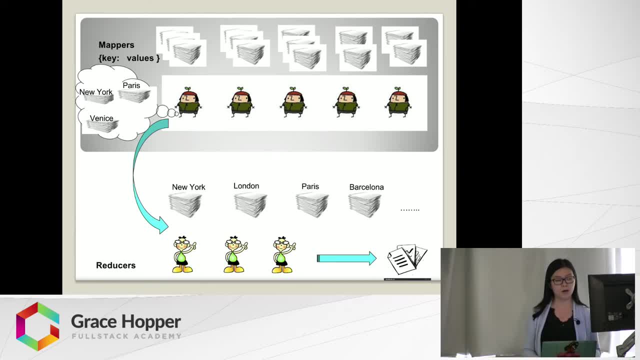 one for London and for all other cities as well. So after they finish this, reducers is going to process the data Like here. we need to calculate the total sales from each city, So they are going to calculate the sales revenue from each city. 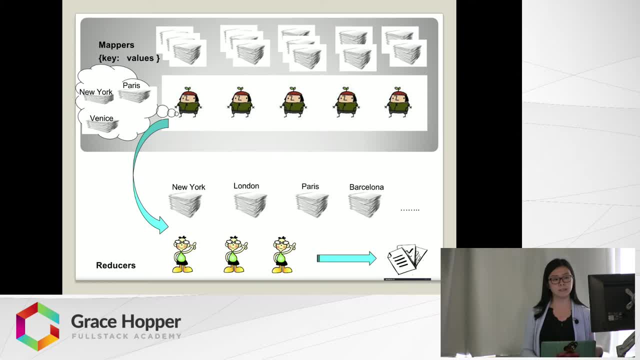 New York, London, one by one and generate the report So we can see from each mapper: here, instead of working on a huge task, they work on a small chunk of task and also they are allowed to work in parallel, which can be very efficient and much faster. 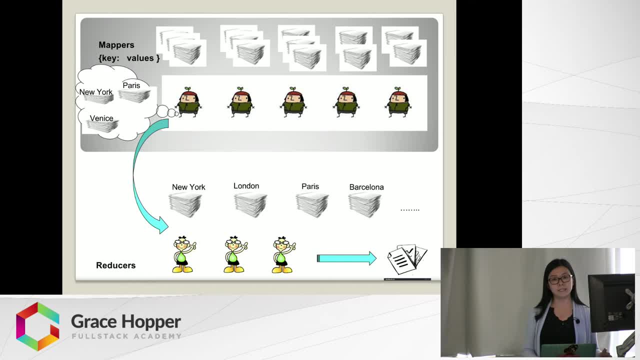 Also, their task is to map all the data into key value pairs. In our case, the key is the name of the city and the value is our transaction data happening in that city. So, for example, I'm going to say New York City. 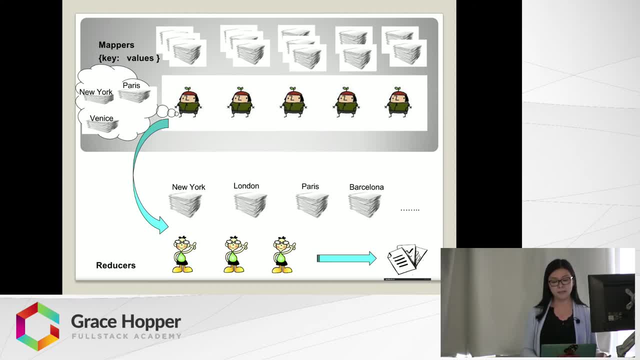 So for reducers, they will get all the data and combine all the values with the same key, Like in our case, our key is the city, So then they are supposed to process the data accordingly, Like here. in our case, we asked them to add up all the sales total for each city.